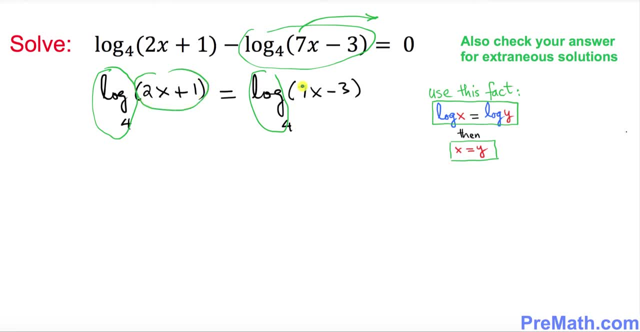 So that means I can say that this part equals to that part. So in other words, I can write as: 2x plus 1 equal to 7x minus 3, using this fact on the right hand side. Now we're going to solve for. 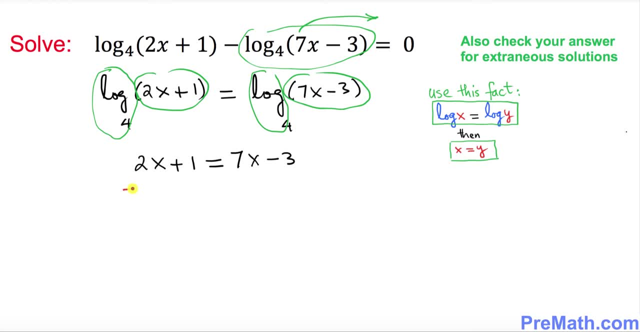 x. So once we solve for x, I'm going to just put down negative 2x on both sides. Okay, so this is gone. So we ended up: 1 equal to 5x minus 3.. I want you to simply add 3 on both sides. So simply, we got. 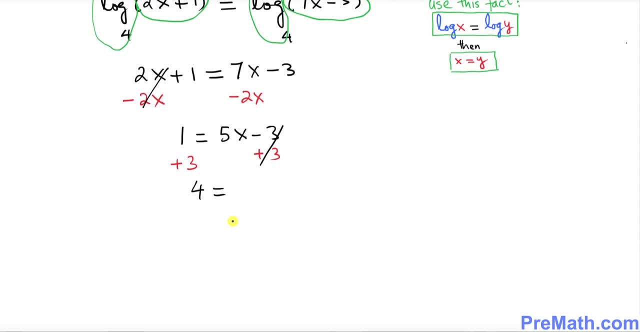 4 equal to 5x, So I want you to divide by 5.. So x turns out to be 4 over 5.. Now the next step is we will take find the extraneous solution And finally, we're going to check our answer for any extraneous solution for this. 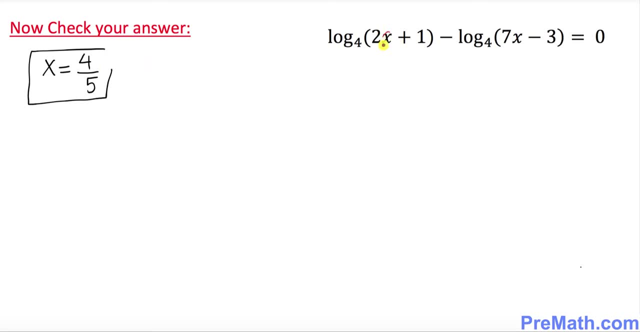 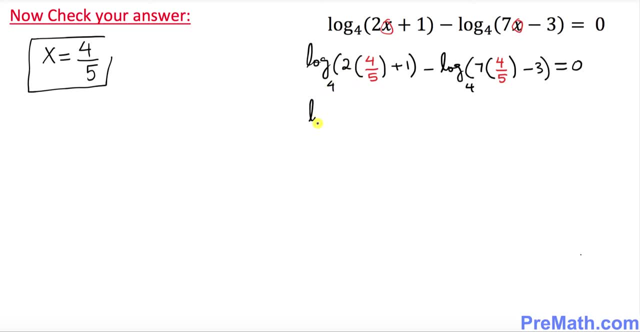 on both sides. Let's go ahead and simplify now. So log of base 4, when you multiply 2 times 4, fifth becomes 8 over 5 plus 1 minus log of base 4.. So I'm going to write the answer down over 5, on the base 4.. This is going to become 28 over 5 minus 3.